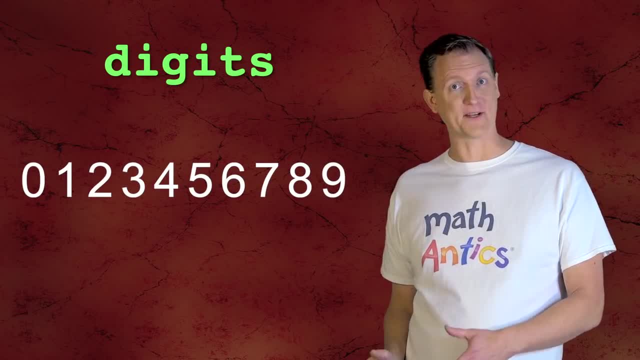 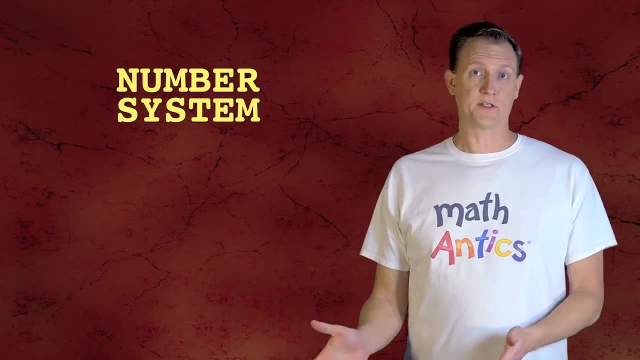 5,, 6,, 7,, 8, and 9.. At first glance you might think that that's only 9 digits, but remember the zero counts as one of the digits, also To see how our number system uses these digits to represent amounts. let's pretend that. 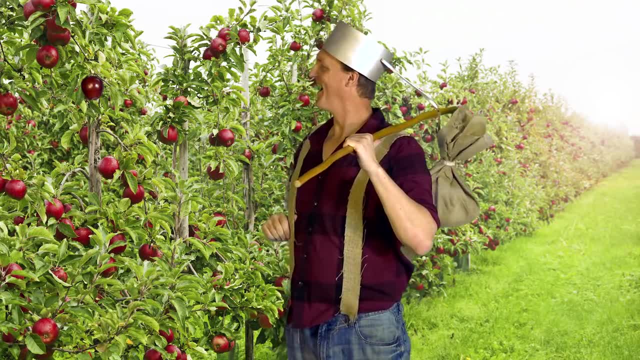 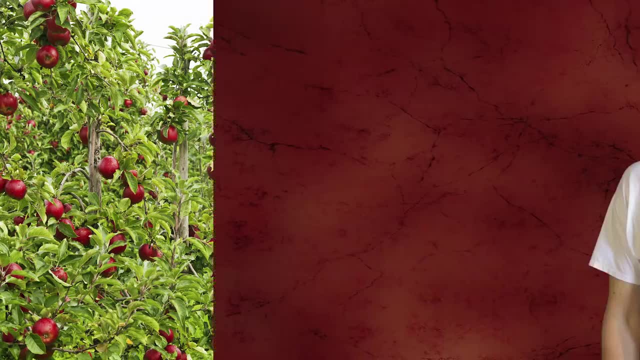 we have an apple orchard full of apple trees And each of these trees is loaded with big, juicy red apples that we need to pick and then count for our records. We're going to use something called a number place to count- The best way to understand. 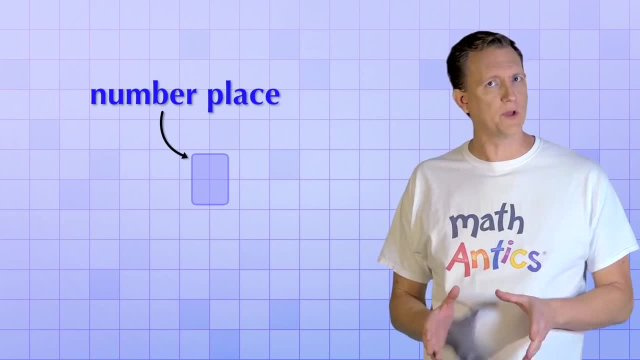 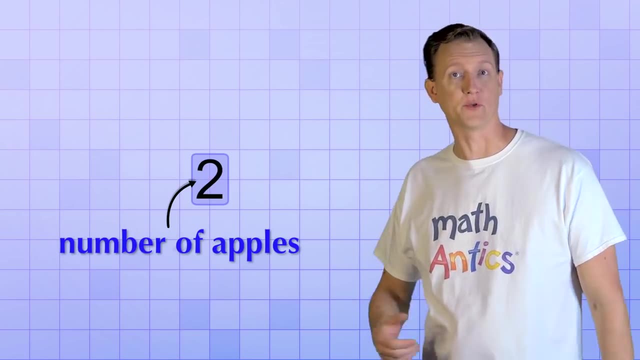 a number place is to imagine that it's like a small box that's only big enough to hold one digit at a time. As we count, we'll change the digit that's in the number place to match how many apples we've picked. For example, if we start with no apples at all, we put the digit 0 in the number place. 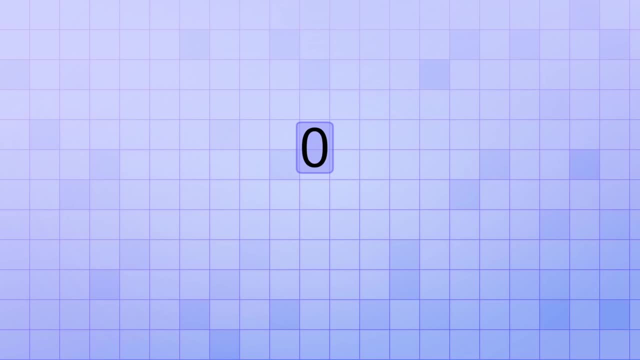 because 0 means none. But then, as the apples start coming in from the orchard, we begin to count: 1,, 2,, 3,, 4,, 5,, 6,, 7,, 8, and 9.. 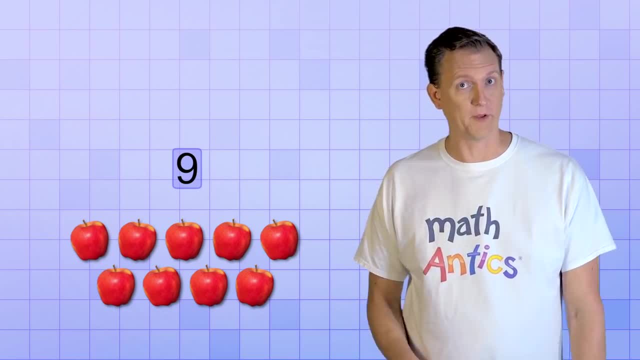 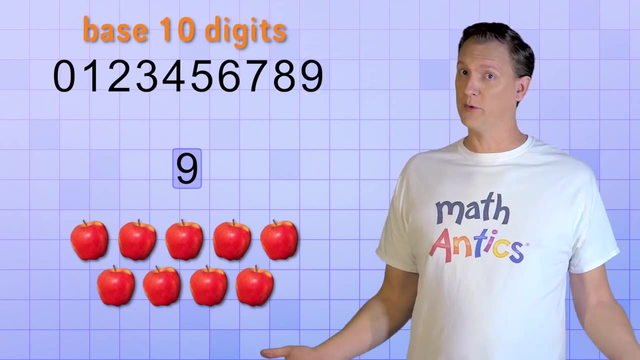 OK, now we've got 9 apples, but we've also got a problem. We've already run out of digits to count, with The highest digit we have is a 9, but there's a lot more apples left to count. What will we do? 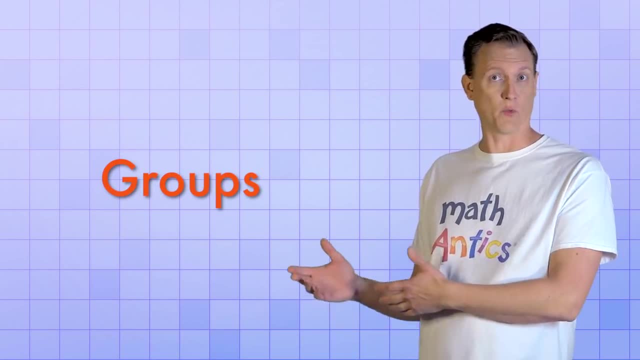 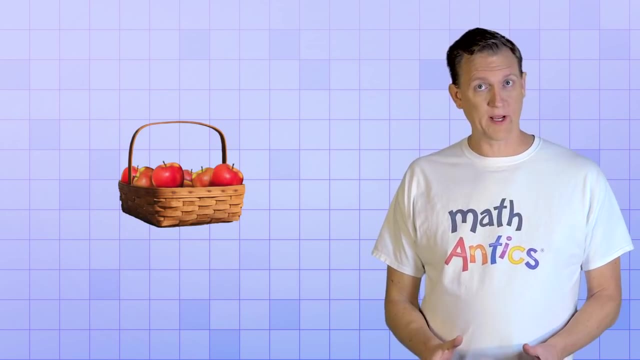 The solution is to use groups to help us count. If we pick just one more apple, we'll have 10, right? So let's combine those 10 apples into a single group. So how many apples do we have 10.. But… how many GROUPS do we have 10.. But… how many? 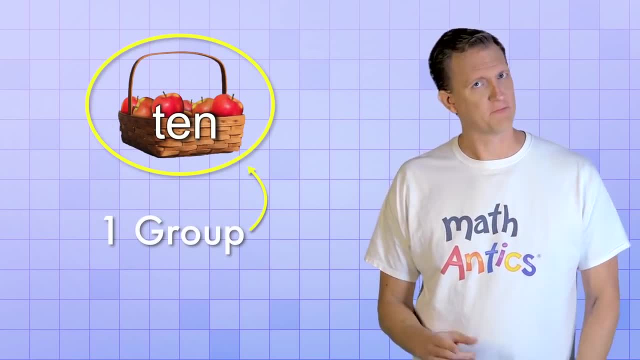 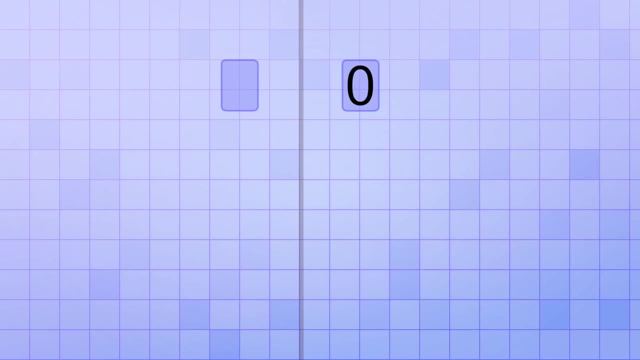 GROUPS of 10 apples. do we have, Ah, just 1.. Does that help us with our lack of digits problem? It sure does… IF we use another number place, Instead of using this new number place, to count up individual apples, one at a time. 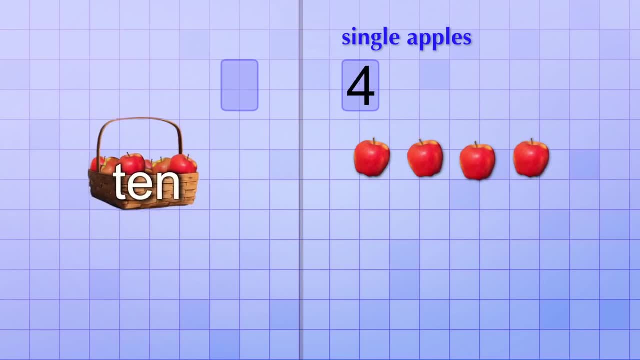 like we did with the first number place, we're going to use it to count apples 10 at a time. In other words, we'll use it to keep track of how many GROUPS of 10 apples that we've picked. For example, if we've picked only 1 group of 10, then we'll put the digit 1 in that. 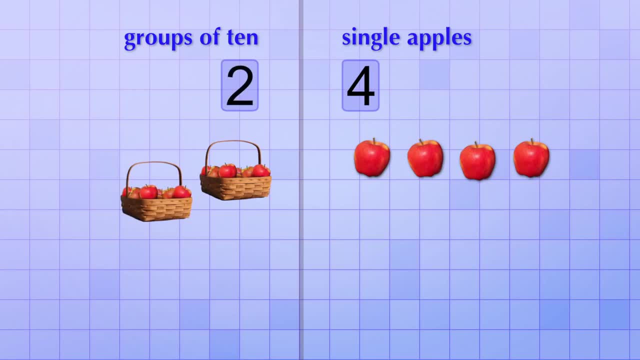 number place. If we've picked 2 groups of 10, then we'll put the digit 2 in that number place, And if we've picked 3 groups of 10, then we'll put the digit 3 in that number place. 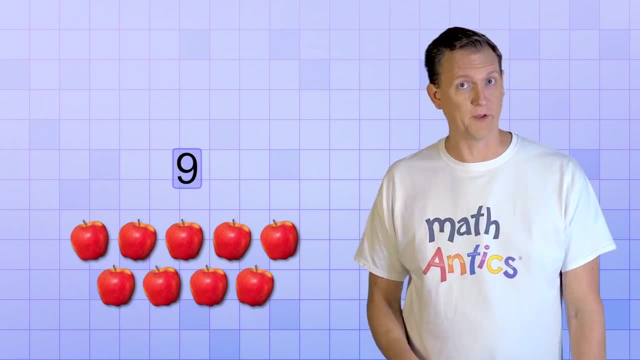 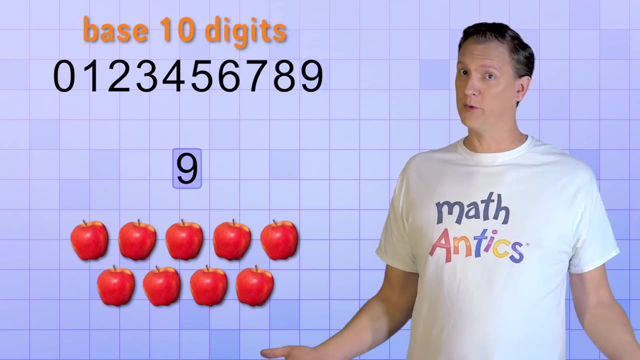 OK, now we've got 9 apples, but we've also got a problem. We've already run out of digits to count with. The highest digit we have is a 9, but there's a lot more apples left to count. What will we do? The solution is to use groups to help us count If we pick. 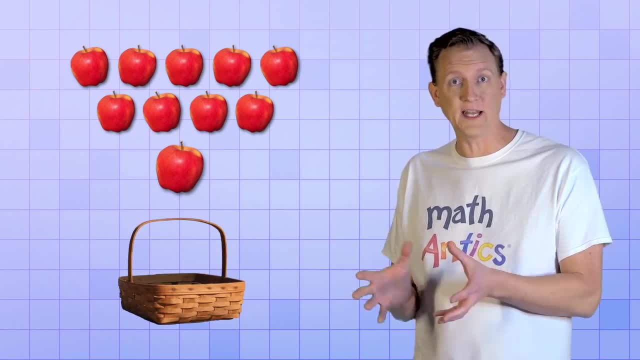 just one more apple, we'll have 10, right? So let's combine those 10 apples into a single group. So how many apples do we have 10.? But… how many apples do we have 10. But… how many. 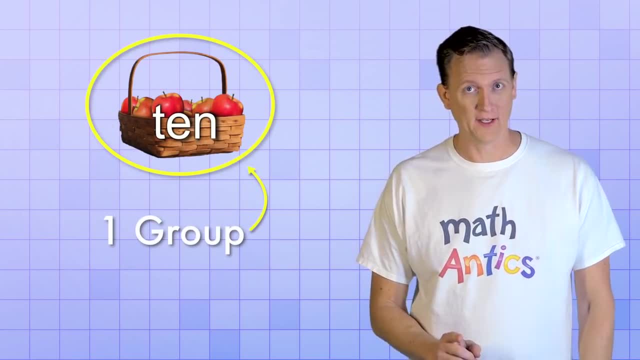 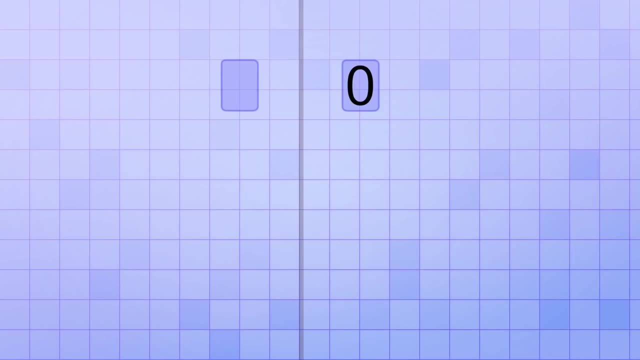 GROUPS of 10 apples. do we have, Ah, just 1.. Does that help us with our lack of digits problem? It sure does… IF we use another number place, Instead of using this new number place, to count up individual apples, one at a time. 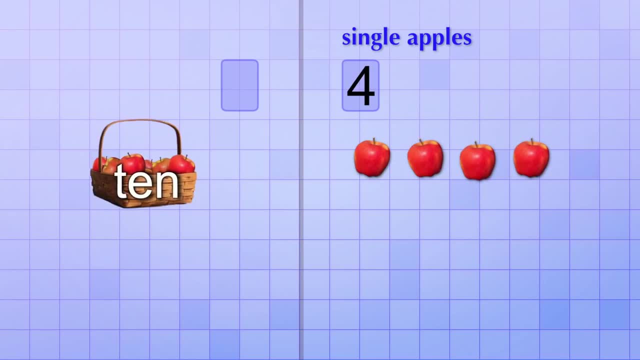 like we did with the first number place, we're going to use it to count apples 10 at a time. In other words, we'll use it to keep track of how many GROUPS of 10 apples that we've picked. For example, if we've picked only one group of 10, then we'll put the digit 1 in that. 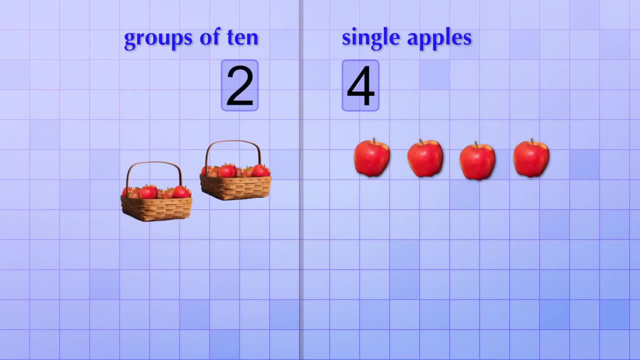 number place. If we've picked only one group of 10, then we'll put the digit 1 in that number place. If we've picked 2 groups of 10, then we'll put the digit 2 in that number place. 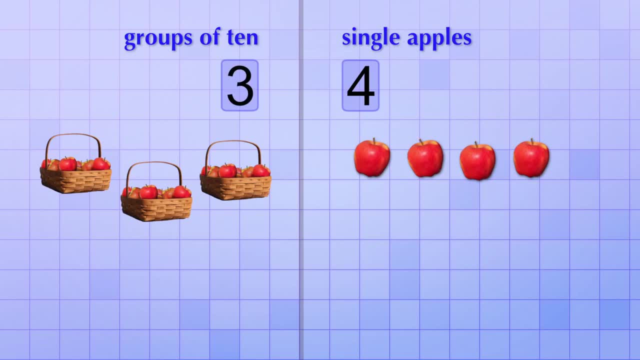 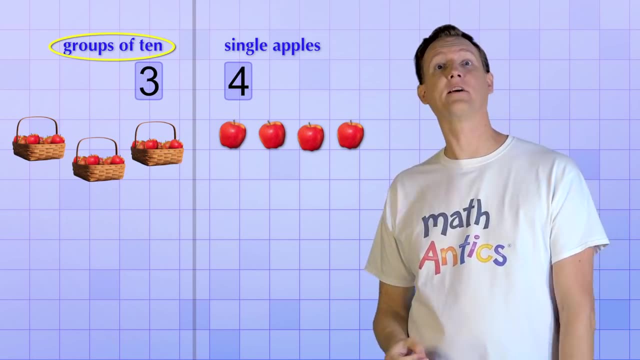 And if we've picked 3 groups of 10, then we'll put the digit 3 in that number place, And so on. Do you see what's happening? Because the new number place is being used to count GROUPS of 10,. it's allowing us to REUSE our original 10 digits, But this time they're able to. 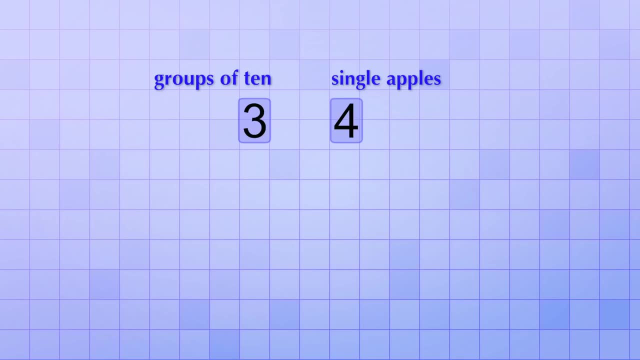 count bigger amounts. Since this new number place is for counting groups of 10, we're going to name it the 10's place, And we'll name our original number place, the 1's place, Because we used it to count things one at a time. 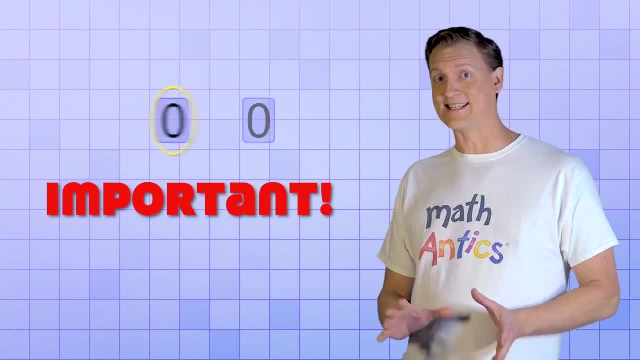 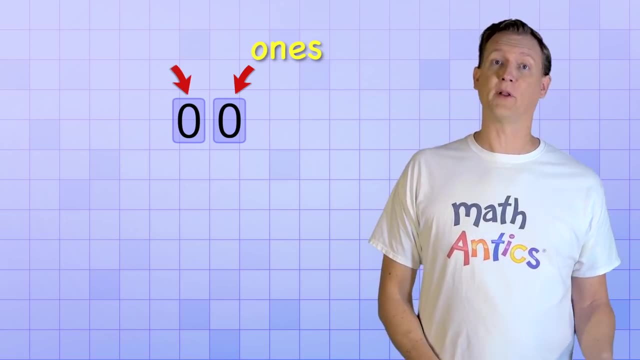 And here's the really important thing: We're not going to use the new number place INSTEAD of the old one. We're going to use it alongside of the old one, so that we have one number place for counting by 1's and another number place for counting by 10's. 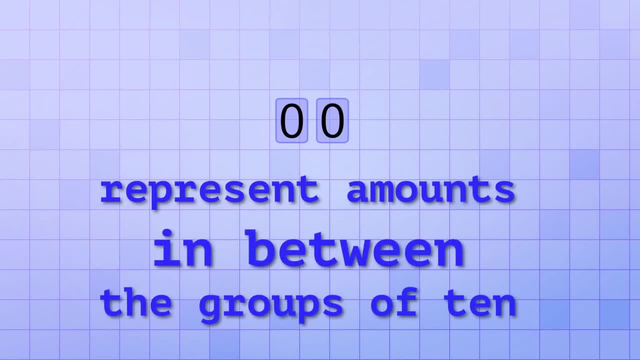 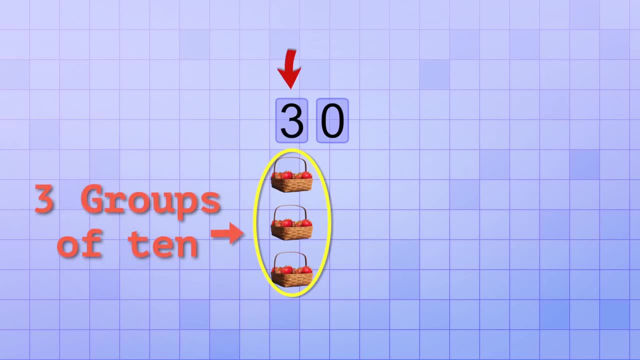 Using these two number places together lets us represent amounts that are IN BETWEEN the groups of 10.. For example, if we've already picked 30 apples, then there'll be a 3 in the 10's place because we have 3 GROUPS of 10.. 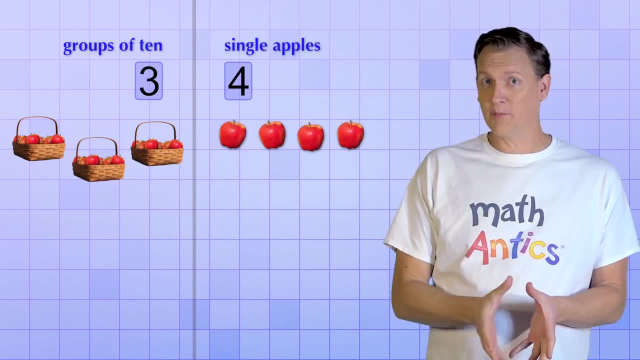 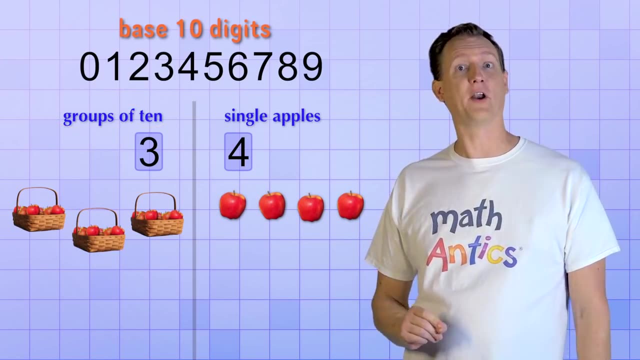 And so on. Do you see what's happening? Because the new number place is being used to count GROUPS of 10, it's allowing us to REUSE our original 10 digits, But this time they're able to count bigger amounts. 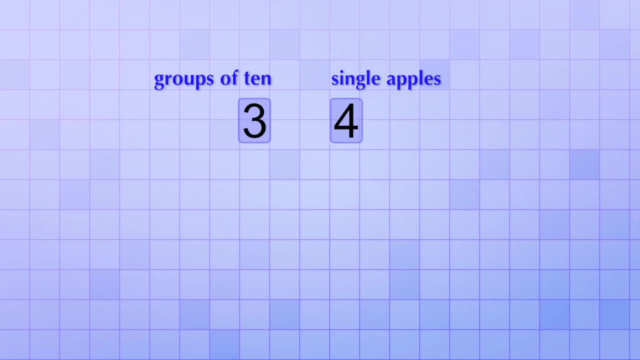 Since this new number place is for counting groups of 10, we're going to name it the 10's place, And we'll name our original number place the 1's place, And we'll name our original number place the 1's place. 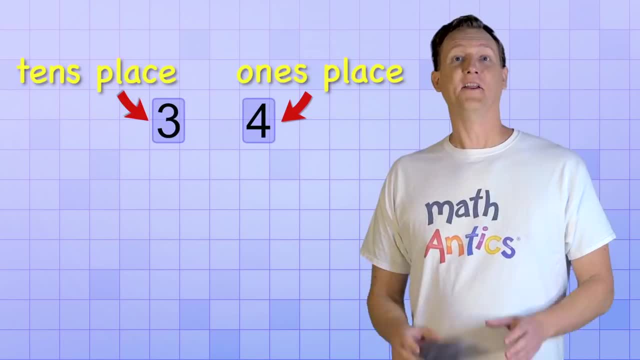 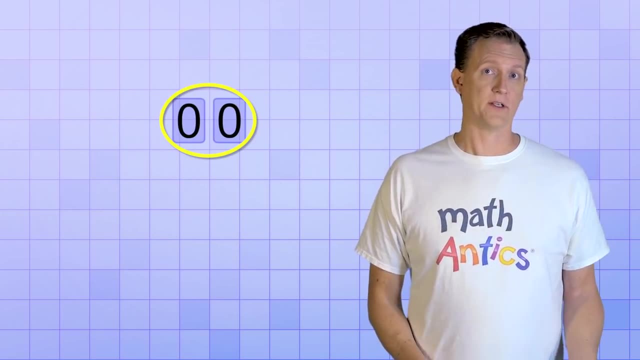 Because we used it to count things one at a time. And here's the really important thing: We're not going to use the new number place INSTEAD of the old one. we're going to use it alongside of the old one, so that we have one number place for counting by 1's. and 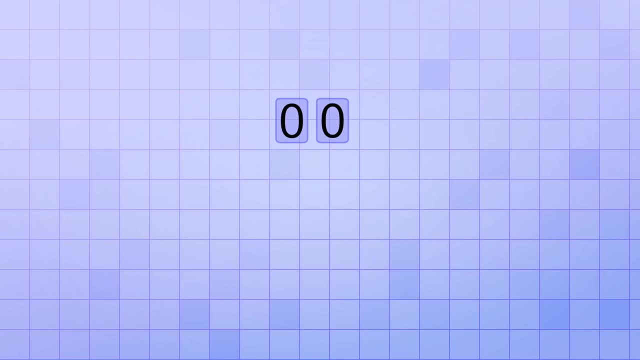 another number place for counting by 10's. Using these two number places together, lets us represent amounts that are IN BETWEEN the groups of 10.. For example, if we've already picked 30 apples, then there'll be a 3 in the 10's place. 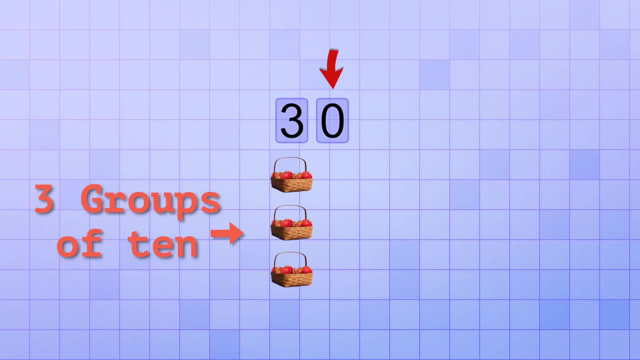 because we have 3 GROUPS of 10. And we'll use these two number places because there are no INDIVIDUAL apples left over. But if we've picked 32 apples, then there'll be a 3 in the 10's place and a 2 in the 1's. 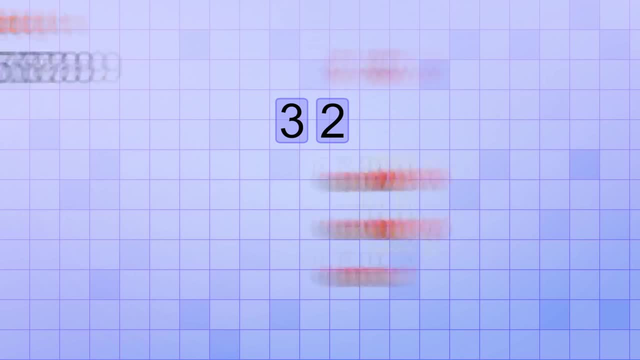 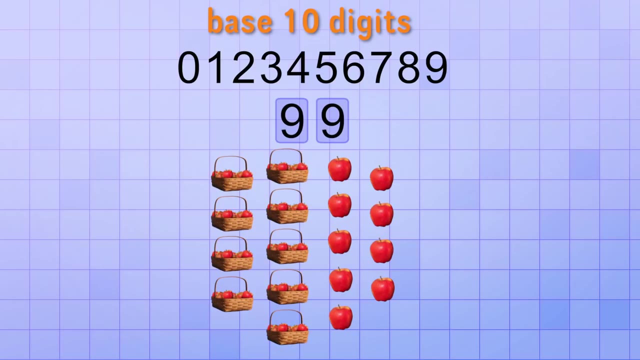 place to represent the 2 individual apples that are NOT in the groups of 10.. In fact, using only our 10 digits and these two number places, we can count all the way from 0 up to 99.. At 99,, both of our number places are maxed out with the HIGHEST digits. 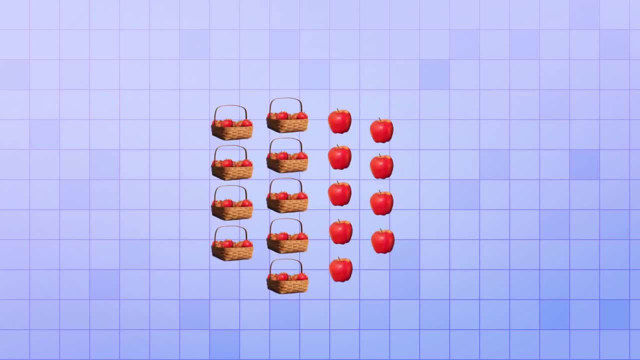 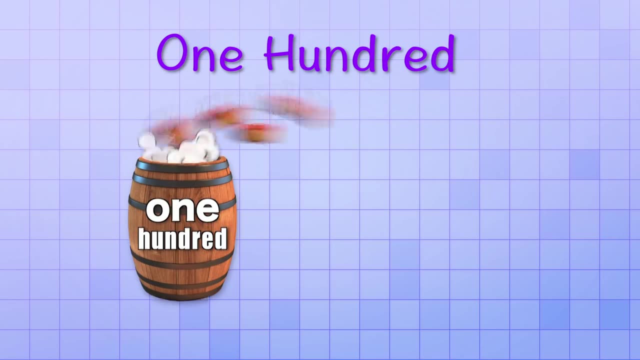 And we won't be able to count any higher… UNLESS… If we pick 99 apples and then we pick just one more, we'll have exactly 100 apples, And if we make a group from those 100 apples, we can use this new number place to count. 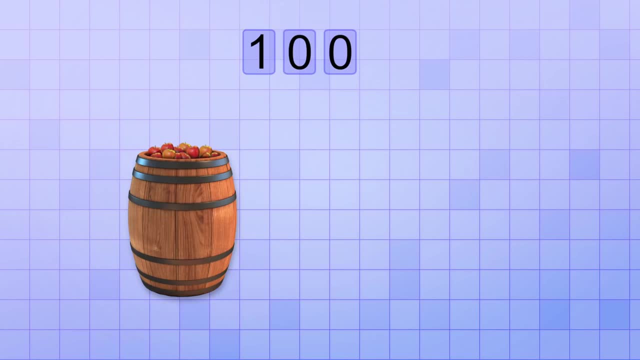 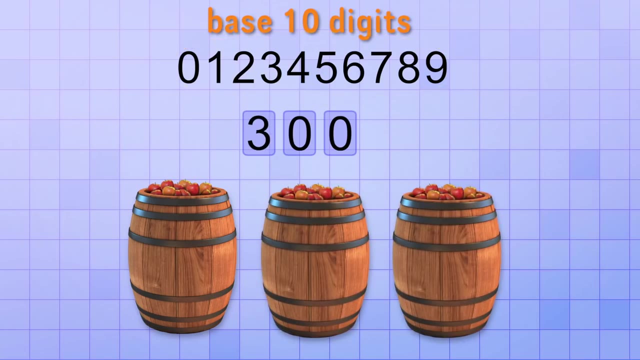 how many groups of 100 we've picked. That means that we can reuse the same 10 digits again in this new number place to count how many groups of 100 we have. And you guessed it, it's called the hundreds place because we use it to count groups of 100. 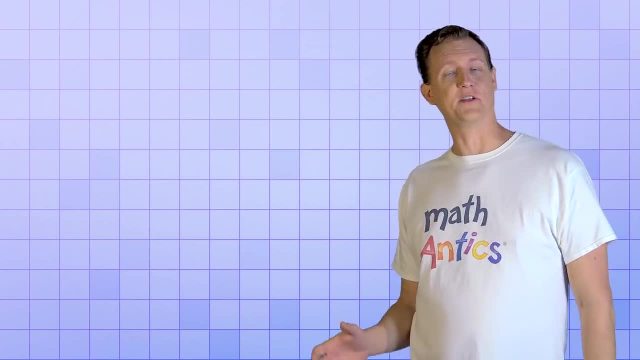 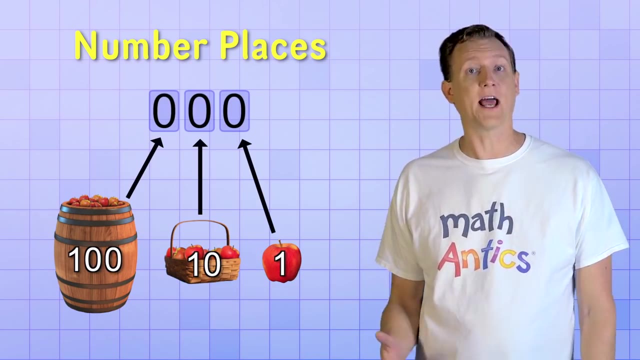 Are you starting to see how our base-10 number system works? It uses different number places to represent the different size groups that we use to count, And the digits in those number places tell us how many of each group we have. The digit in the ones place tells us how many ones we have. 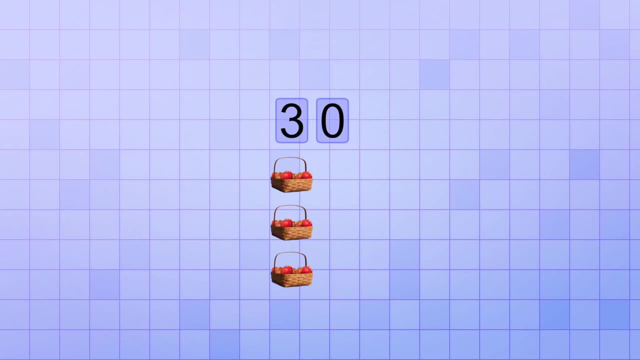 And if we've picked 32 apples, then there'll be a 3 in the 10's place and a 2 in the 1's place to represent the 2 individual apples that are not in the groups of 10.. In fact, using only our 10 digits and these two number places, we can count all the way. 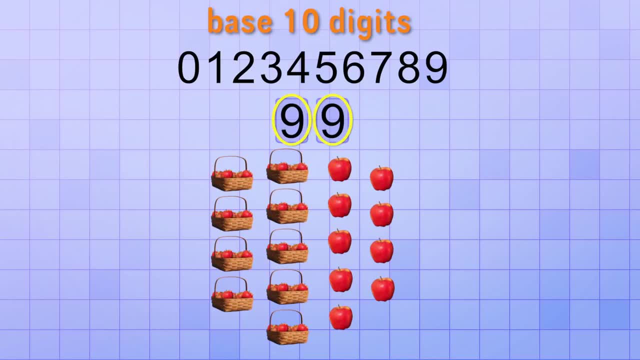 from 0 up to 99.. At 99,, both of our number places are maxed out with the highest digits And we won't be able to count any higher unless we get another number place. But if we've picked 32 apples, then there'll be a 3 in the 10's place and a 2 in the 1's. 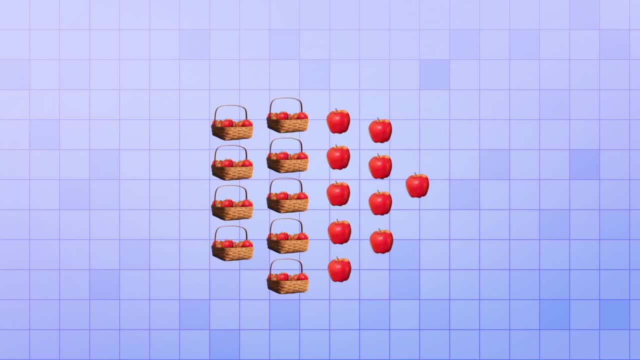 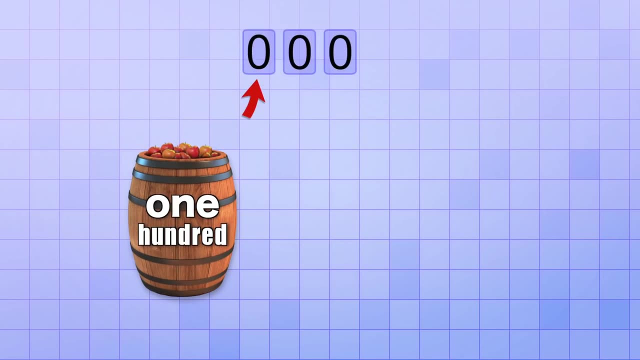 place. If we've picked 99 apples and then we pick just one more, we'll have exactly 100 apples, And if we make a group from those 100 apples, we can use this new number place to count how many groups of 100 we've picked. 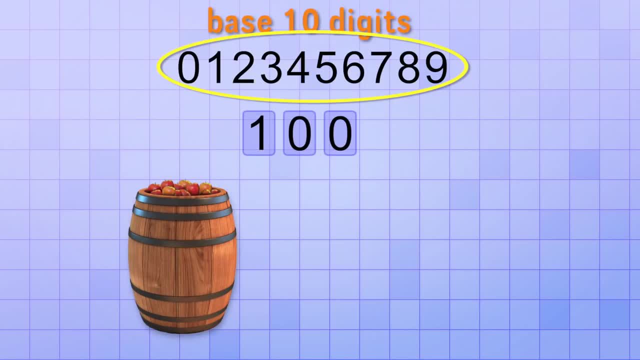 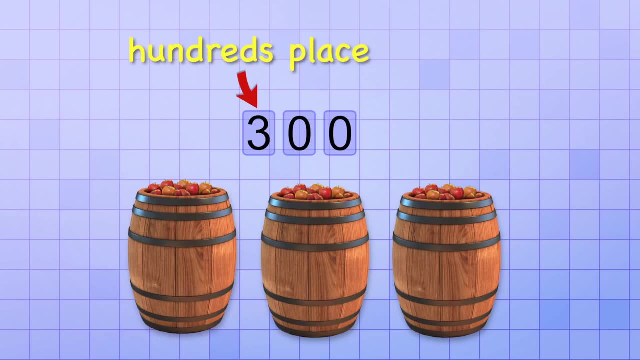 That means that we can reuse the same 10 digits again in this new number place to count how many groups of 100 we have. And you guessed it: it's called the 100's place because we use it to count groups of 100.. 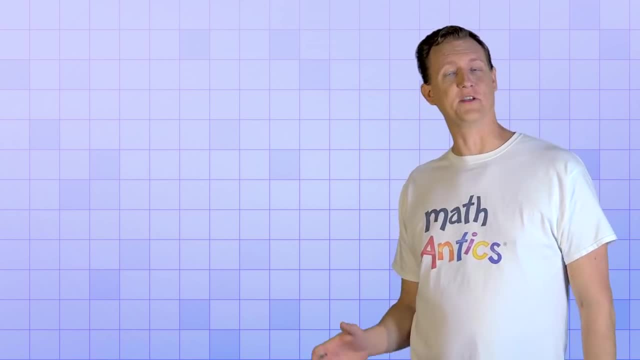 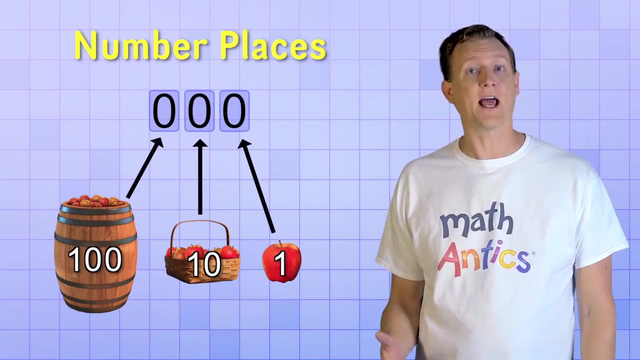 Are you starting to see how our base 10 number system works? It uses different number places. It uses different number places to represent the different size groups that we use to count, And the digits in those number places tell us how many of each group we have. 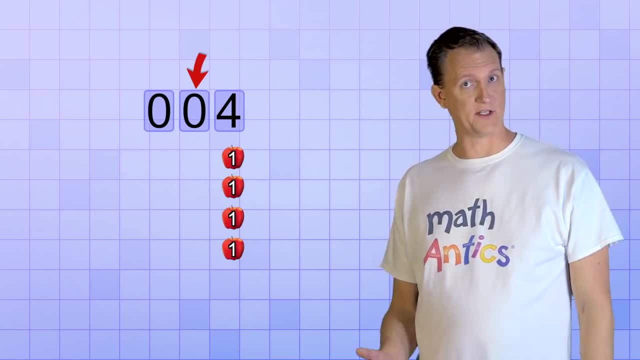 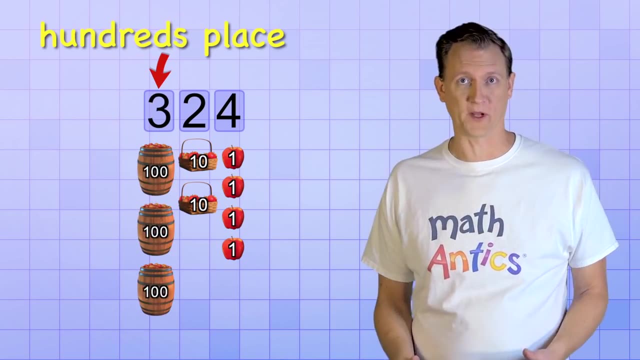 The digit in the 1's place tells us how many 1's we have. The digit in the 10's place tells us how many groups of 10 we have, And the digit in the 100's place tells us how many groups of 100 we have. 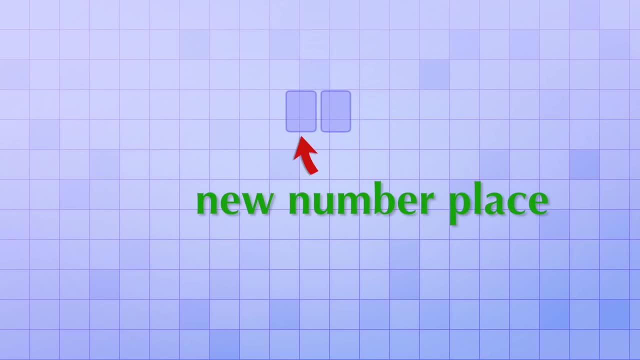 And have you noticed that each time we got a new number place to count larger groups, we placed it to the left of the previous number place? That's important Because number places are always arranged in the exact same order, Starting with the 1's place. as you move to the left, the number places represent larger. 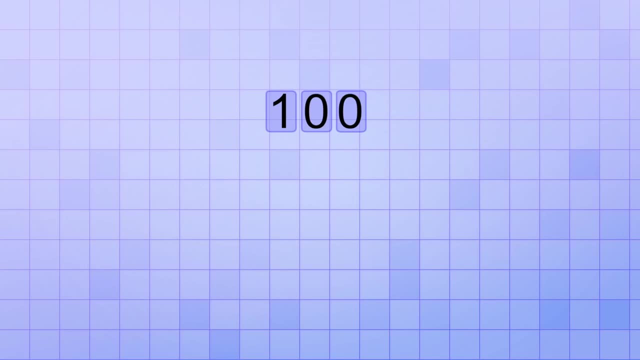 and larger amounts? And did you also notice that each new number place represents groups that are exactly 10 times bigger than the previous number place? 10 is 10 times bigger than 1 and 100 is 10 times bigger than 10.. 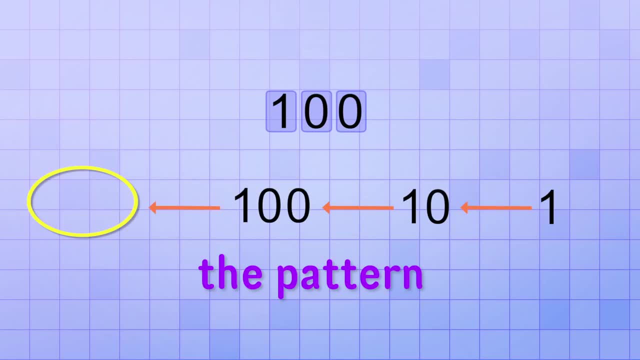 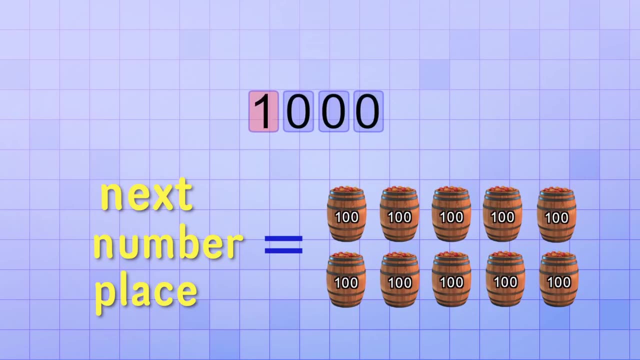 That's really important because it helps us see the pattern for even bigger number places. It helps us to see that the next number place will count groups of 10 times 100. Which is 1000. And that's why it's called the 1000's place. 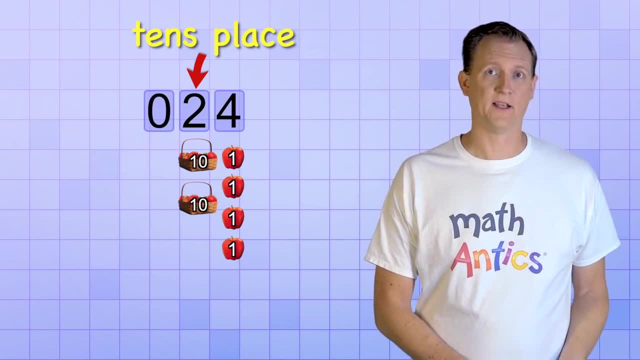 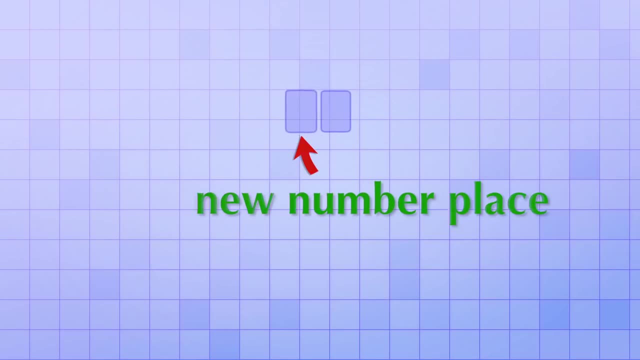 The digit in the tens place tells us how many groups of 10 we have, And the digit in the hundreds place tells us how many groups of 100 we have. And have you noticed that each time we got a new number place to count larger groups? 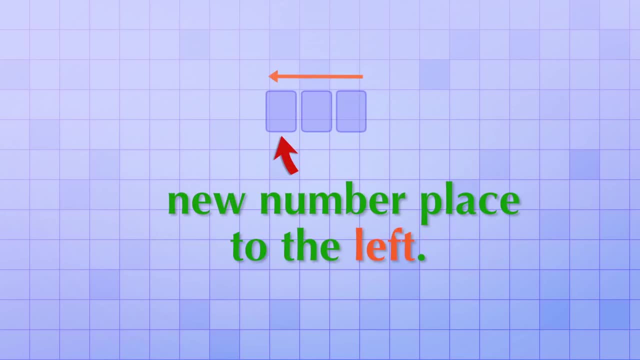 we placed it to the left of the previous number place. That's important, Because number places are always arranged in the exact same order, Starting with the ones place. as you move to the left, the number places represent larger and larger amounts. And did you also notice that each new number place represents groups that are exactly 10? 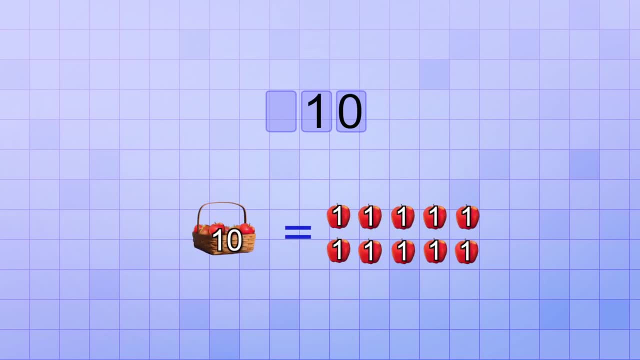 times bigger than the previous number place. 10 is 10 times bigger than 1 and 100 is 10 times bigger than 10.. That's really important because it helps us see the pattern for even bigger number places. It helps us to see that the next number place. 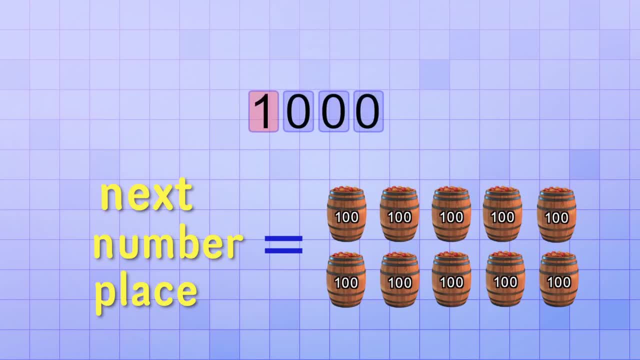 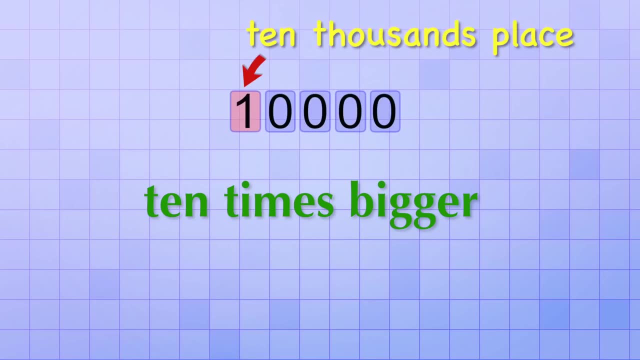 will count groups of 10 times 100,, which is 1000.. That's why it's called the thousands place, And the next number place will count groups 10 times bigger than that. It's the ten thousands place. And the number places keep on going like that. 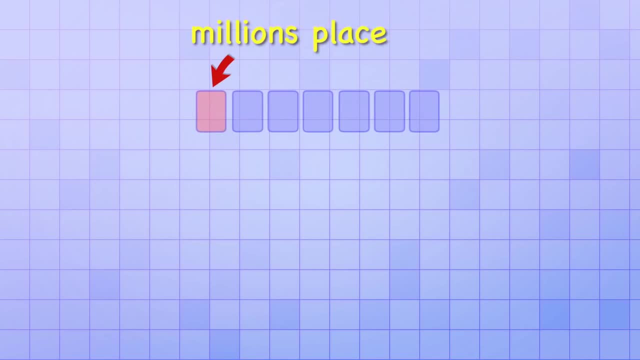 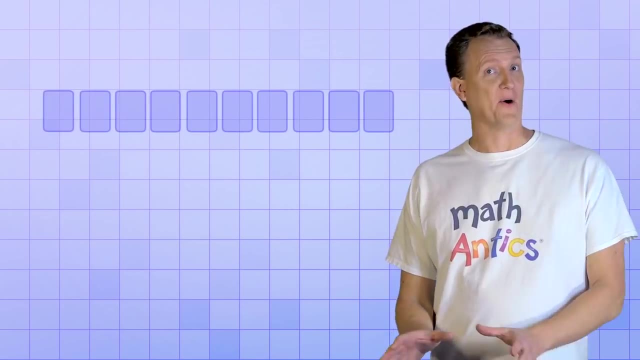 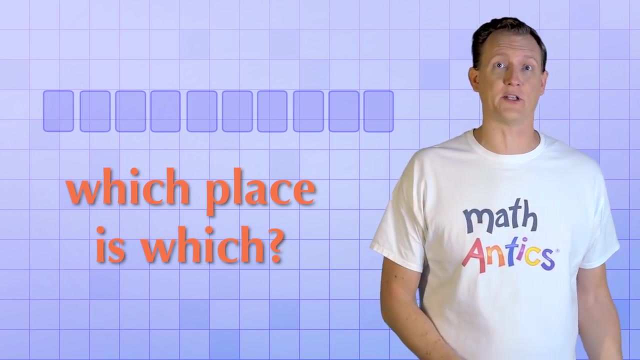 Next is the hundred thousands place, Then the millions place, Then ten millions, Then a hundred millions, Then billions, And so on. Oh, and you may notice that when we get a lot of number places next to each other like this, it's a little hard to quickly recognize which place is which. 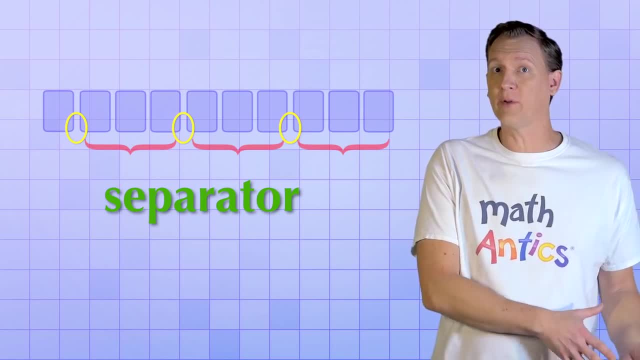 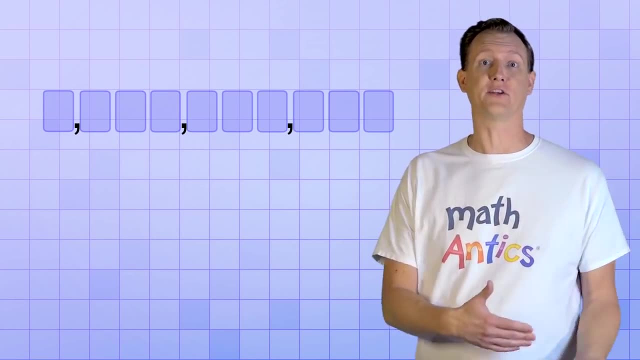 That's why many countries use some kind of separator every three places to make them easier to keep track of. For example, in the US we use a comma every three number places to make it easier to identify things like the thousands place or the millions place. 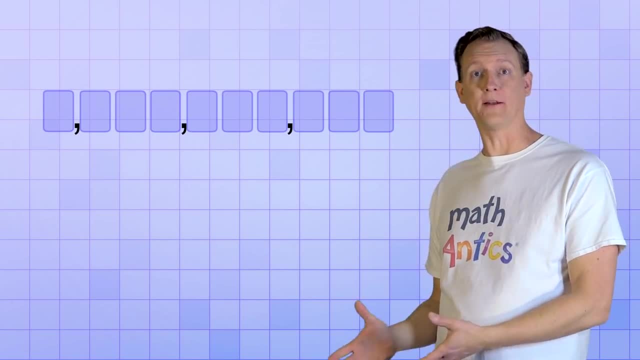 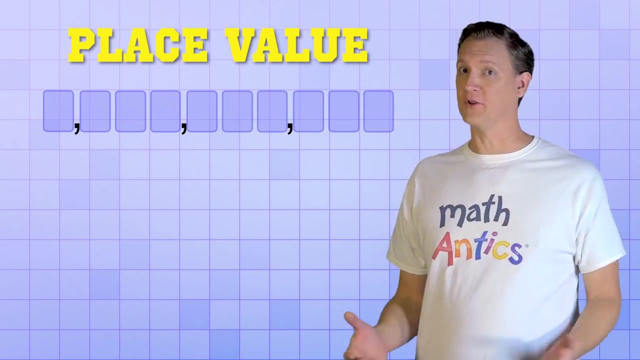 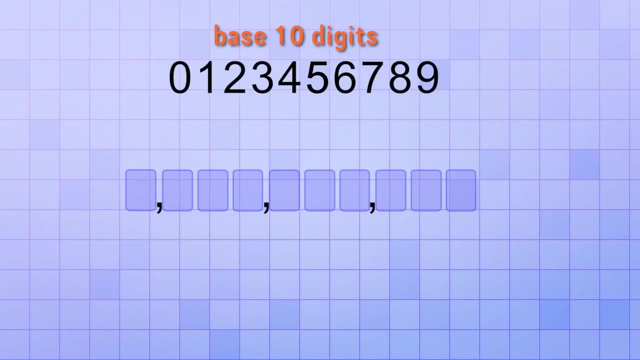 Seeing all these number places together helps you understand what we mean by place value. In a multi-digit number, the number place that a digit is in determines its value. Even though we only have 10 digits, each digit can stand for different amounts depending on the place that it occupies. 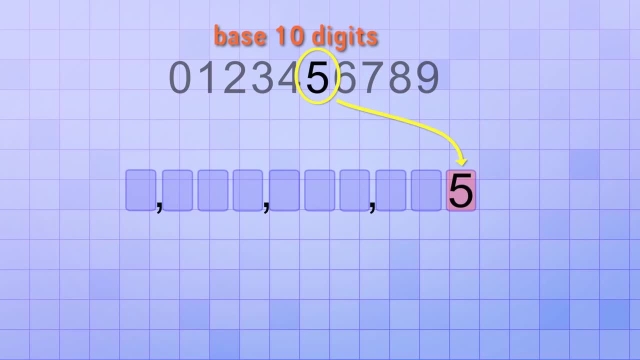 If the digit 5 is in the ones place, it just means 5.. But if a 5 is in the tens place, then it means 50. And if a 5 is in the hundreds place it means 500. And it's the same for bigger number places. 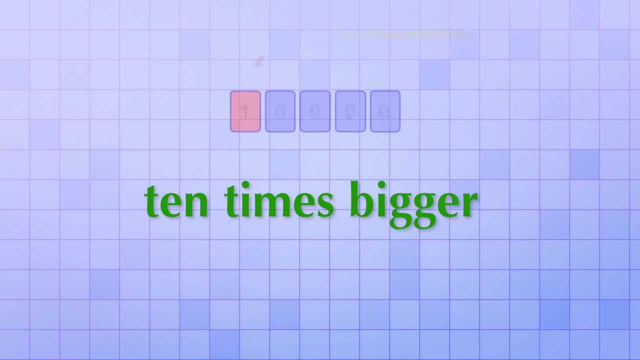 And the next number place will count groups 10 times bigger than that. It's the 10,000's place, And the number places keep on going like that. Next is the 100,000's place, Then the million's place. 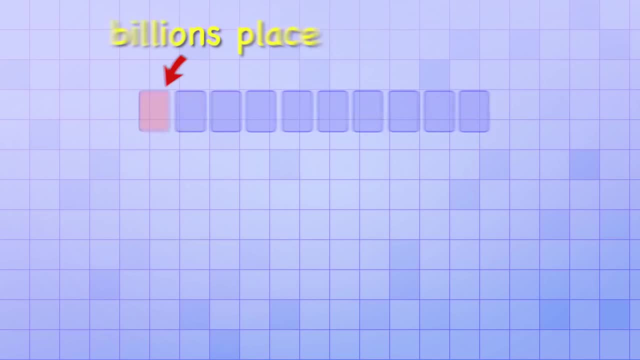 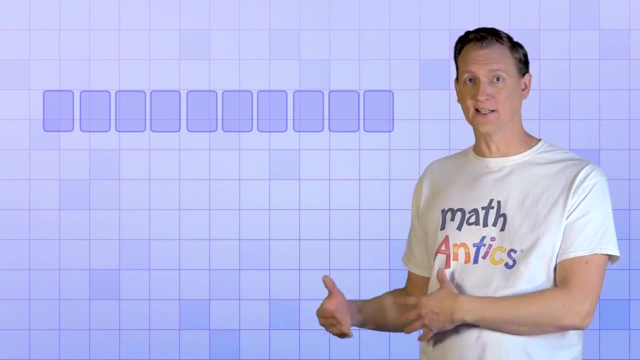 Then 10 million's, Then 100 million's, Then billion's, And so on. Oh, and you may notice that when we get a lot of number places next to each other like this, it's a little hard to count them all together. 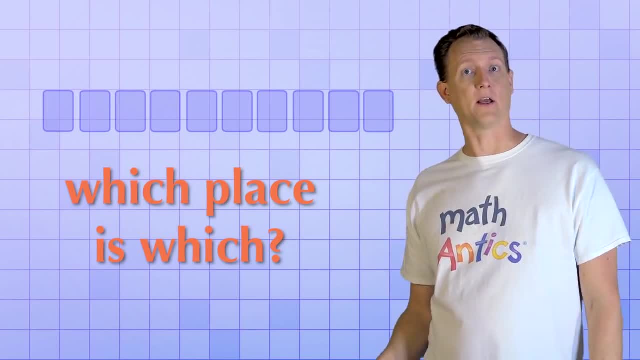 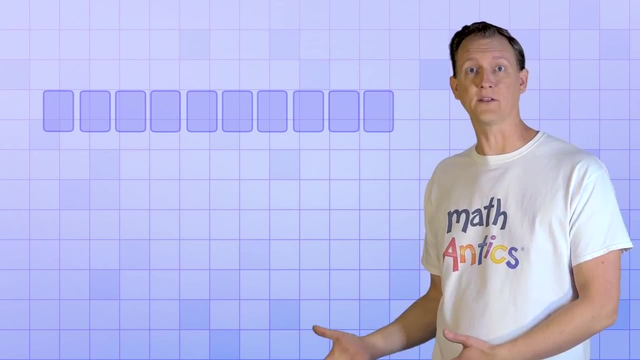 It's hard to quickly recognize which place is which. That's why many countries use some kind of separator every 3 places to make them easier to keep track of. For example, in the US we use a comma every 3 number places to make it easier to identify. 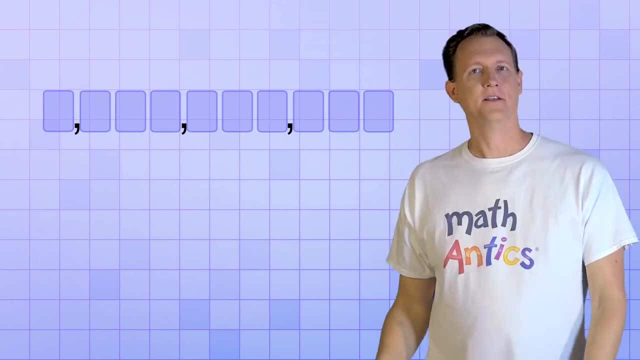 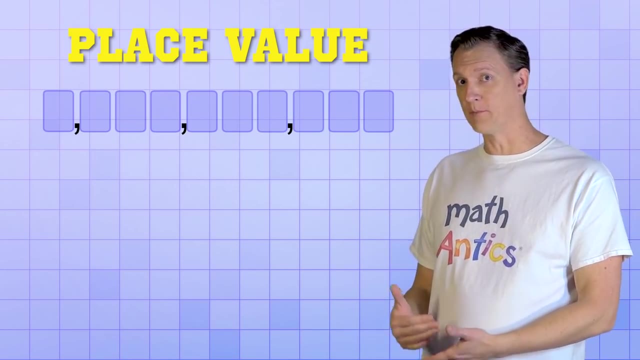 things like the 1000's place or the million's place. Seeing all these number places together helps you understand what we mean by place value. In a multi-digit number, the number place that a digit is in determines its value, Even though we only have 10 digits. 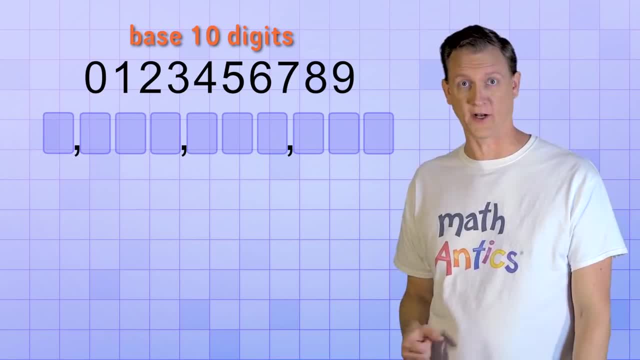 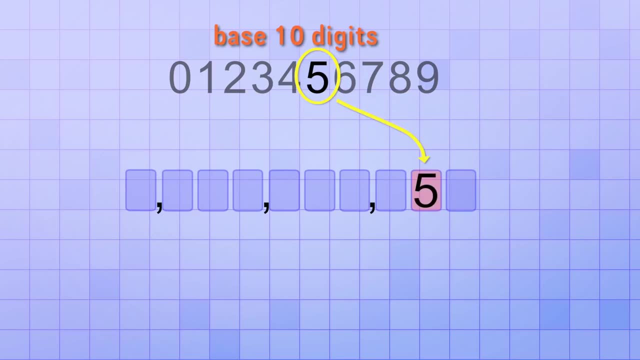 each digit can stand for different amounts depending on the place that it occupies. If the digit 5 is in the 1's place, it just means 5.. But if a 5 is in the 10's place, then it means 50.. 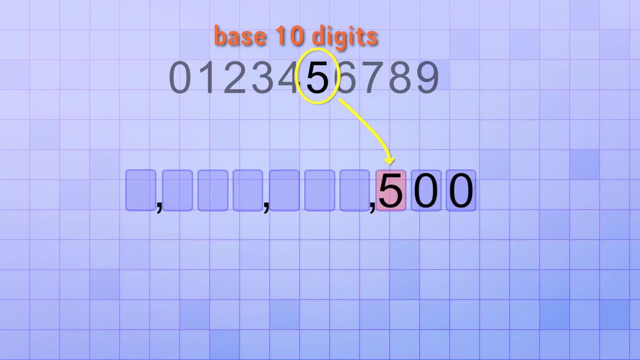 And if a 5 is in the 100's place, it means 500. And it's the same for bigger number places. A 5 in the 100,000's place means 500,000. And a 5 in the billion's place means 5 billion. 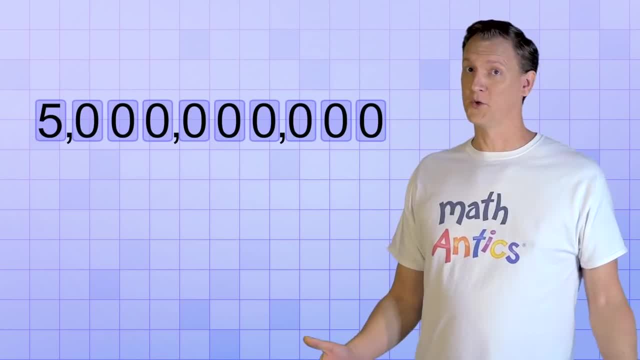 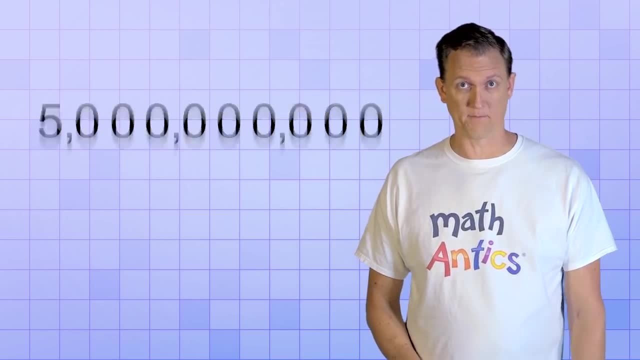 See how a digit's place affects its value. Of course, When you're studying numbers in math, most of the time the number places are invisible, But the underlying pattern is always the same. Oh, and because the number places are invisible, in certain cases you'll need to use zeros. 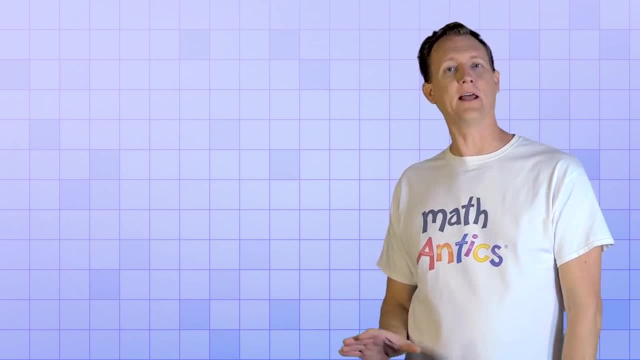 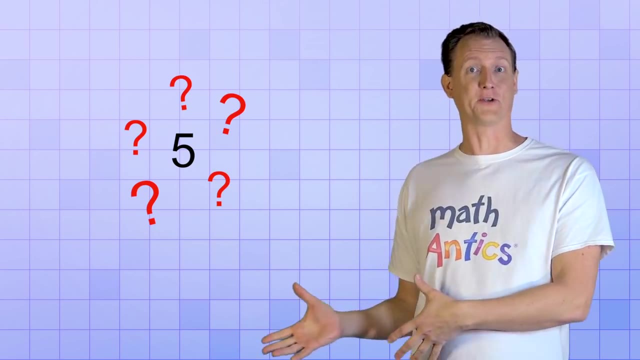 to make it clear what number you're talking about. To see what I mean, imagine that this 5 is in the 100's place to represent 500. But if you make the number places invisible, then it just looks like 5 and not 500.. 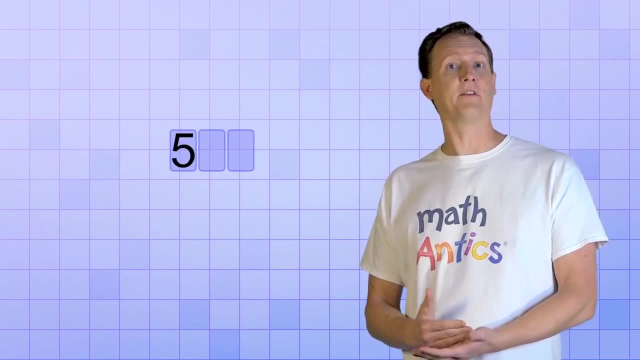 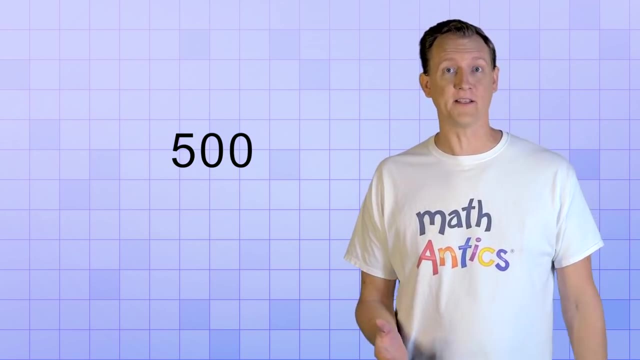 So to make sure people know you mean 500, you need a 5 in the 100's place, a 0 in the 10's place and a 0 in the 1's place. Now you can tell that the 5 is in the 100's place and it means 500. 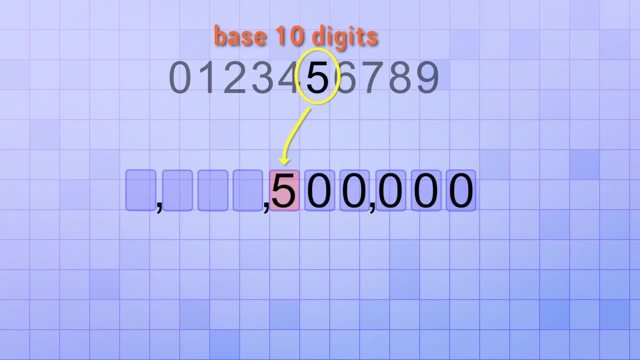 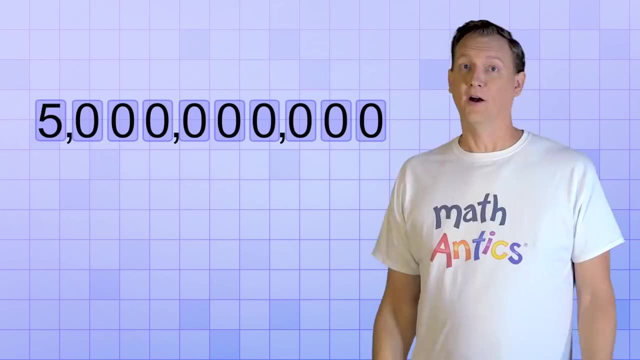 A 5 in the hundred thousands place means 500,000.. And a 5 in the billions place means 5 billion. See how a digit's place affects its value. Of course, when we work with numbers in math, most of the time the number places are invisible. 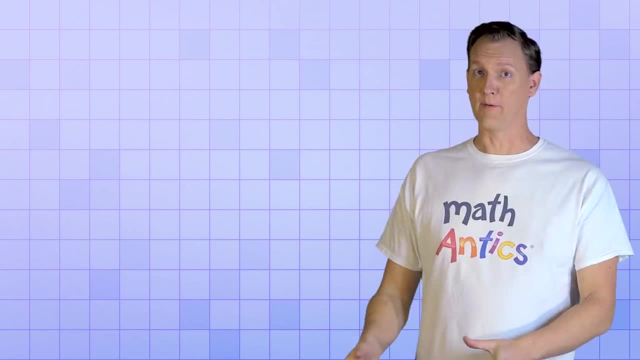 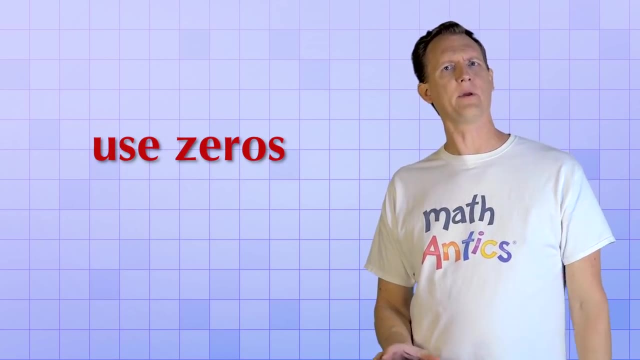 But the underlying pattern is always the same. Oh, and because the number places are invisible, in certain cases, you'll need to use zeros to make it clear what number you're talking about. To see what I mean, imagine that this 5 is in the hundreds place to represent 500.. 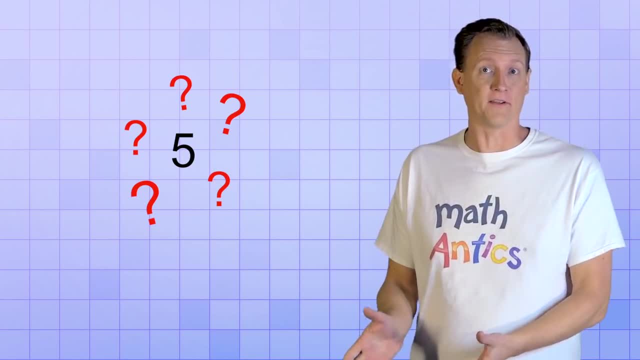 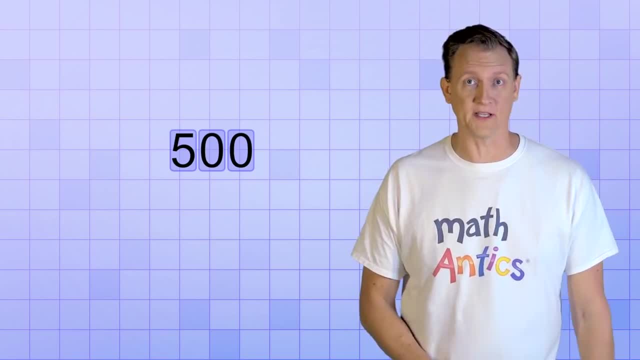 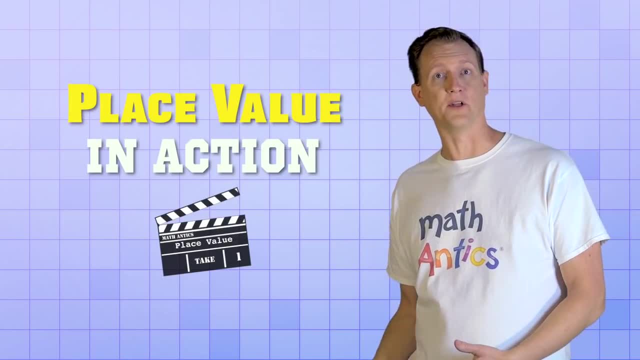 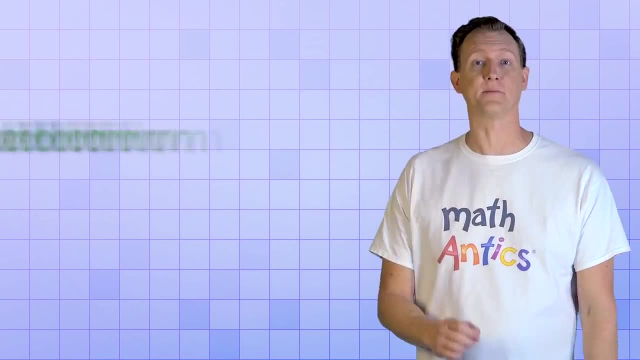 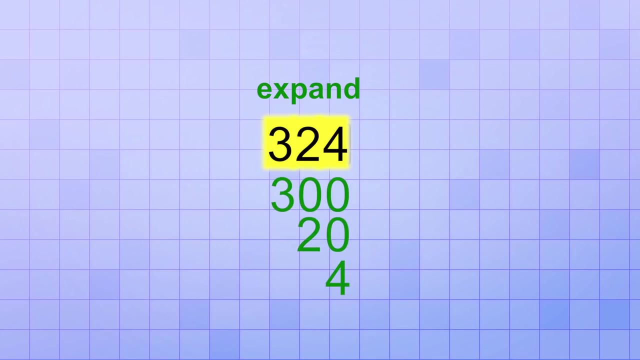 Okay now. a great way to see place value in action with some actual numbers is to expand them to show that they're really combinations of different groups. When we do this, it's called writing a number in expanded form. For example, we can expand 324 to be 300,, 20 and 4. 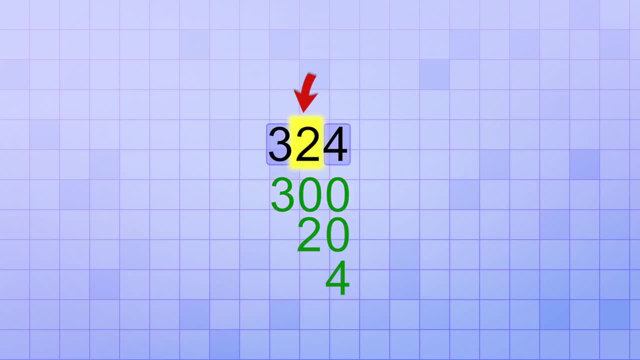 because the 3 is in the hundreds place and means 300,, the 2 is in the tens place and means 20, and the 4 is in the ones place, so it just means 4.. So 324 in expanded form is the combination of those amounts. 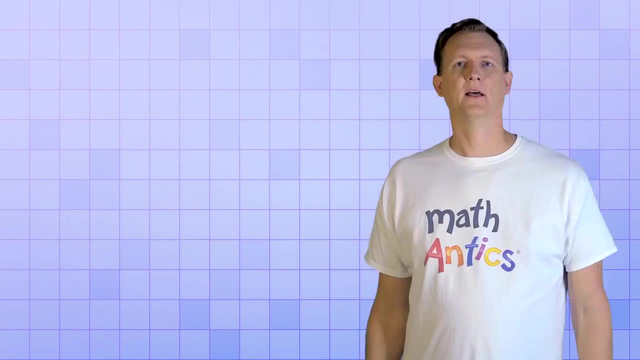 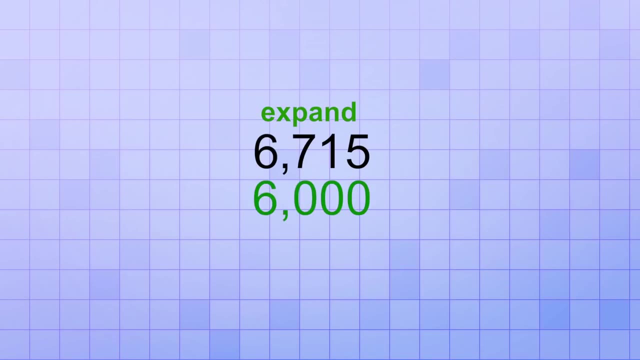 300 plus 20 plus 4.. Let's try writing another number in expanded form: 6,715.. We can expand this into 6,000, because the 6 is in the thousands place, plus 700, because the 7 is in the hundreds place. 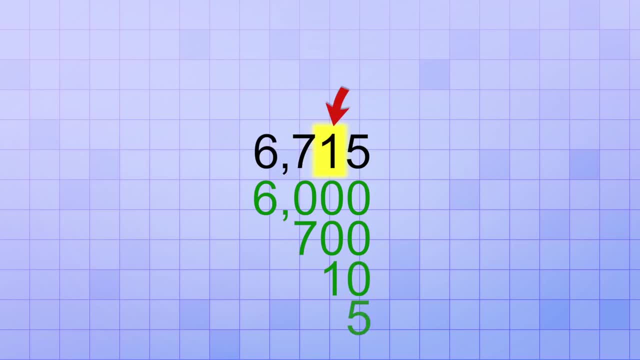 plus 10, because the 1 is in the hundreds place and 5 because the 5 is in the ones place. So the expanded form is 6,000 plus 700 plus 10 plus 5.. Alright, so do you see how our base 10 number system works.